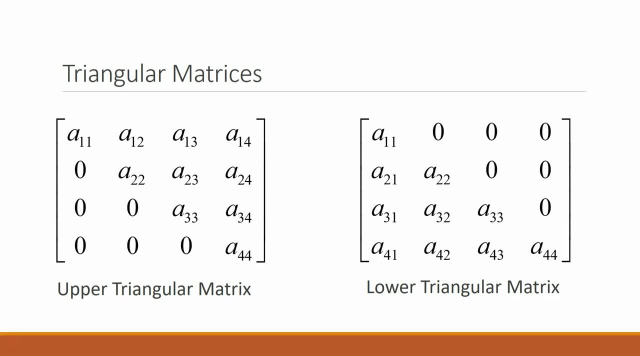 which there are only zeros above or below the main diagonal. A matrix which contains elements above or on the main diagonal is considered an upper triangular matrix, as seen here on the left, and a matrix where its elements are below or on the main diagonal is considered a. 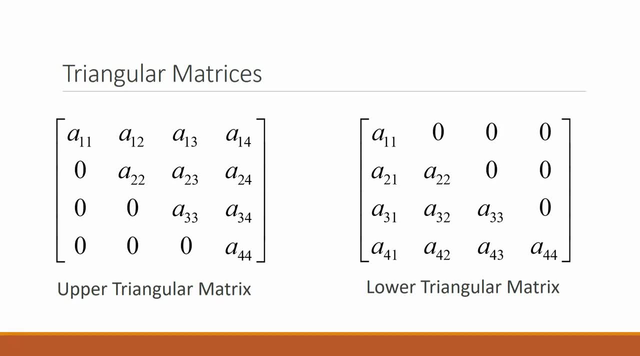 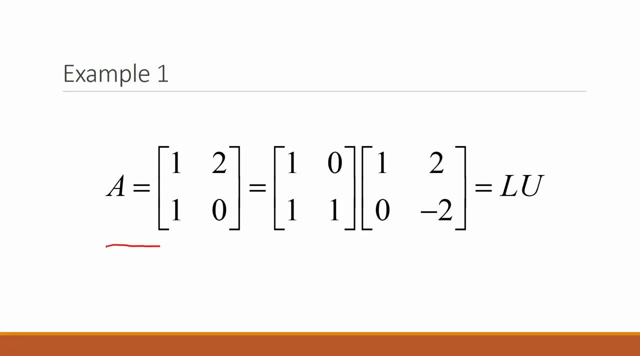 lower triangular matrix, as seen here on the right In example 1, we are given a matrix A, which equals 1, 2, 1, 0, which can be split into two separate matrices, one upper triangular and one lower triangular. L represents the lower triangular matrices and U represents the upper triangular matrices We can show. 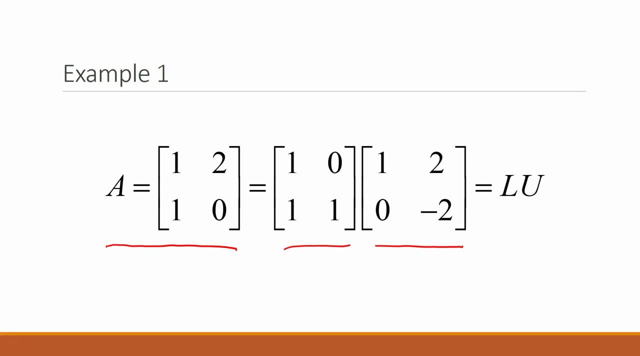 that L times U is the lower triangular matrix and U is the upper triangular matrix. So we can see that L times U equals A. By computing a simple matrix multiplication between L and U, we can see that the product of the upper and lower triangular matrices equals A. our given 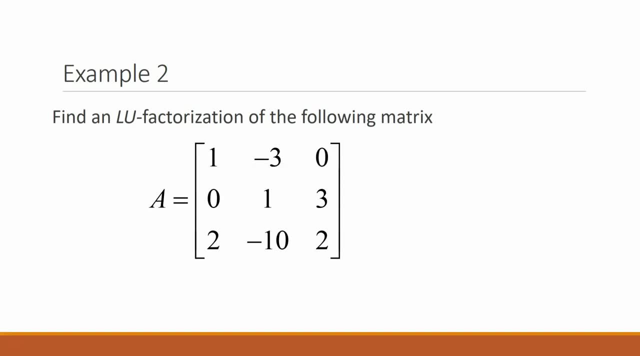 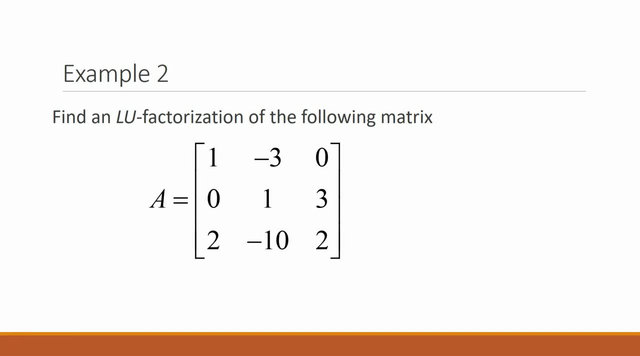 We can find the triangular matrices through the use of Gaussian elimination Example: 2. Find an LU factorization of the following matrix A: Notice: we start by setting up our paper with a designated place in the upper right-hand corner to begin building matrix L: 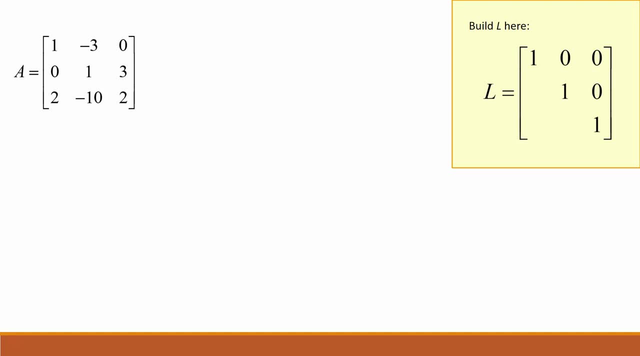 Begin by trying to reduce A into an upper triangular matrix. Begin with this number 2 in row 3.. What elementary operation could we apply to make this 2 into a 0? Multiply row 1 by negative 2 and add it to row 3 to get a new row 3.. 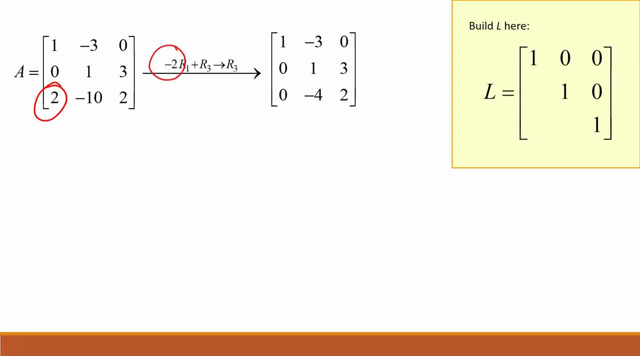 Since we multiplied by a negative 2, to turn this 2 into a 0, we will take the opposite of negative 2 and place it in the corresponding area in our L-matrix 2.. Now, what elementary operation could we apply to make this negative 4 into a 0?? 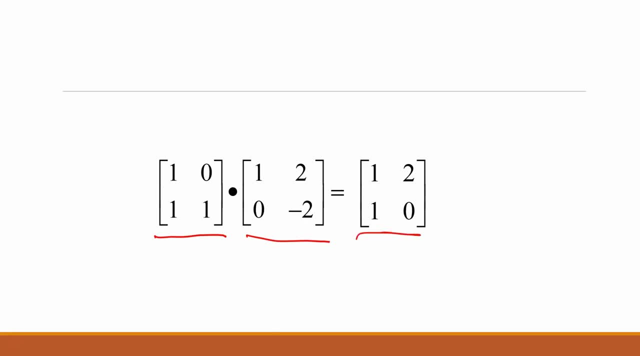 triangular matrices equals A, our given. In example one we saw that L times U equals A. but the question remains: how do we determine the matrices L and U? We can find the triangular matrices through the use of Gaussian elimination Example. 2.. Find an LU factorization of the following matrix A: 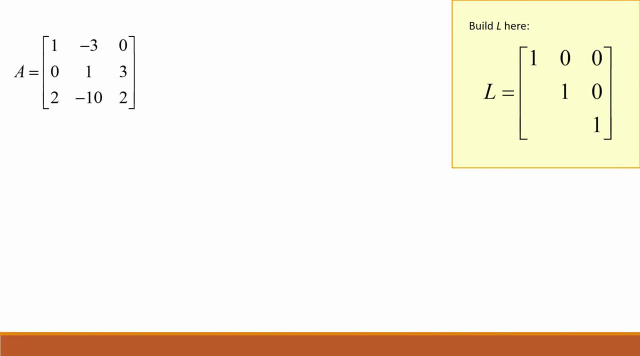 Notice. we start by setting up our paper with a designated place in the upper right-hand corner to begin building matrix L. Begin by trying to reduce A into an upper triangular matrix. Begin with this number 2 in row 3.. What elementary operation could we apply to make this 2 into a 0?? 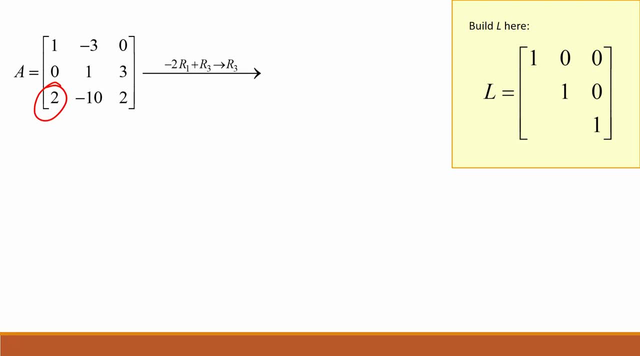 Multiply row 1 by negative 2 and add it to row 3 to get a new row 3.. Since we multiplied by a negative 2 to turn this 2 into a 0, we will take the opposite of negative 2 and place it in the corresponding area in our L-matrix 2.. 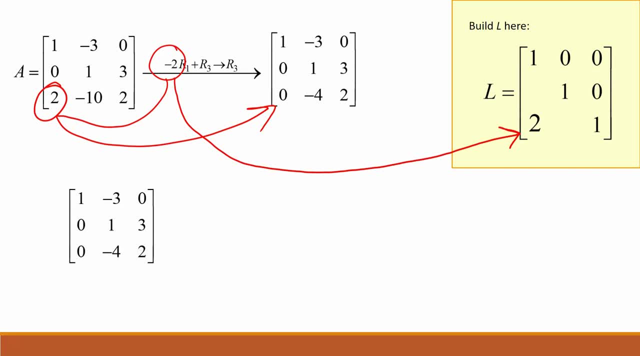 Now what elementary operation could we apply to make this negative 4 into a 0?? Multiply row 2 by 4 and add it to row 3 to get a new row 3.. Since we multiplied by a positive 4 to turn this negative 4 into a 0,. 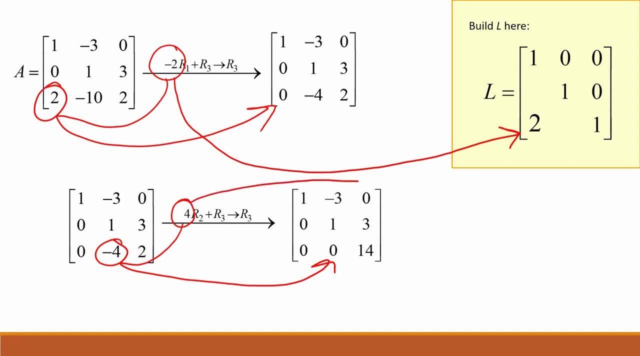 we will take the opposite of 4 and place it in the corresponding area of our L-matrix 2.. Now what elementary operation could we apply to make this negative 4 into a 0? Multiply row 2 by 4 and add it to row 3 to get a new row 3.. Since we multiplied by a negative 4, to turn this negative 4 into a 0,, we will take the opposite of 4 and place it in the corresponding area in our L-matrix 2.. Since we multiplied by a negative 4, to turn this negative 4 into a 0,. we will take the opposite of 4 and place it in the corresponding area in our L-matrix 2.. Since we multiplied by a negative 4 to turn this negative 4 into a 0, we will take the opposite of 4 and place it in the corresponding area in our L-matrix 2.. Since we multiplied by a negative 4, to turn this negative 4 into a 0,, we will take the opposite of 4 and place it in the corresponding area in our L-matrix 2.. Since we multiplied by a negative 4, to turn this negative 4 into a 0,. 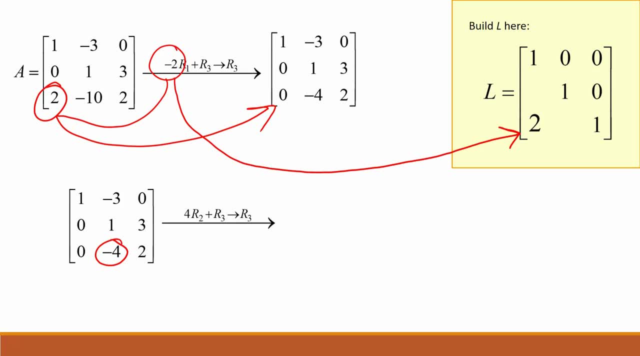 Multiply row 2 by 4 and add it to row 3 to get a new row 3.. Since we multiplied by a positive 4 to turn this negative 4 into a 0, we will take the opposite of 4 and place it in the corresponding area of our L-matrix 2.. 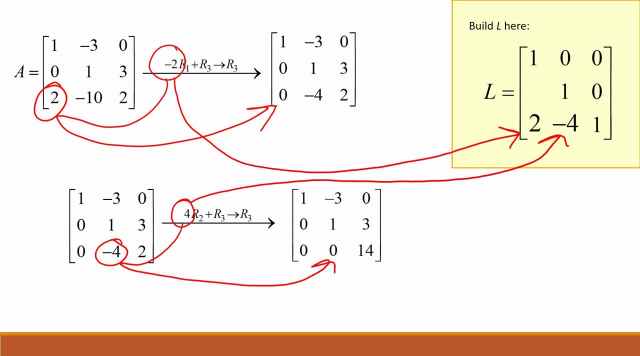 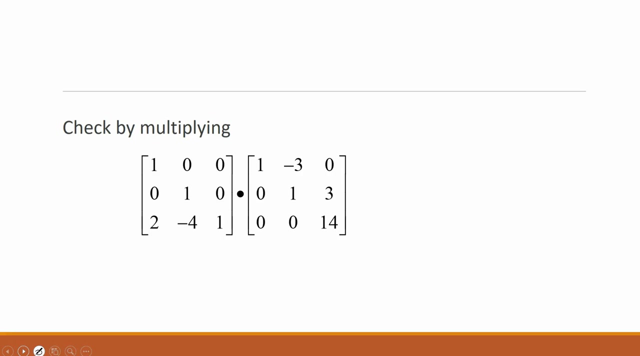 Now what elementary operation could we apply to make this negative 4 into a 0? queue? Multiply row 2 by 4 and add it to row 3 to get a new row and a new matrix multiplication. we see the product of L and U is equal to our original matrix A. 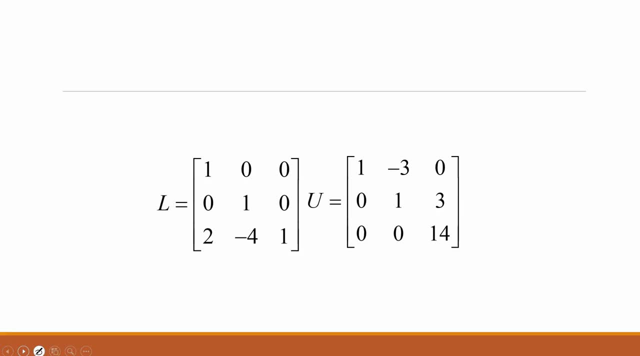 This would be the final answer for the LU factorization of matrix A. LU factorization can be utilized to solve a system of equations. We are given this linear system. If we convert this to a non-augmented matrix, the result is: 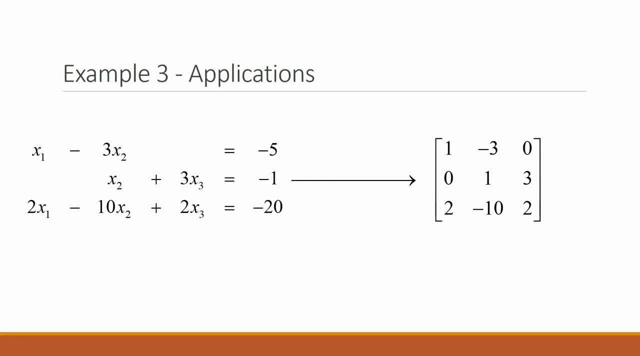 This matrix should look familiar because it is the same matrix as in example two. Step one: The first step in solving a linear system using LU factorization is to compute LU factorization. We factored A in example two and these were our L and U. 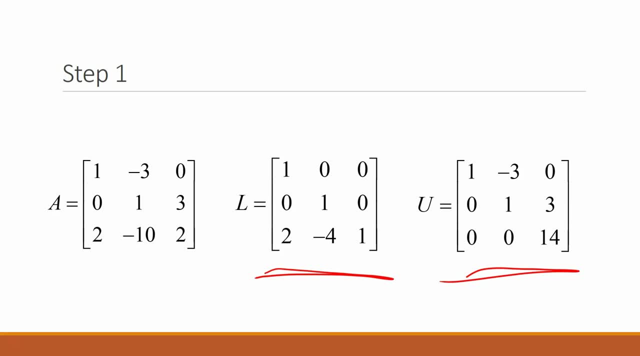 matrices which we will use. for example, three: Step two: Let L times Y equal B and solve for Y- L is our lower triangular matrix- times Y equals B, which are the answers to the linear system. The goal of step two is to solve. 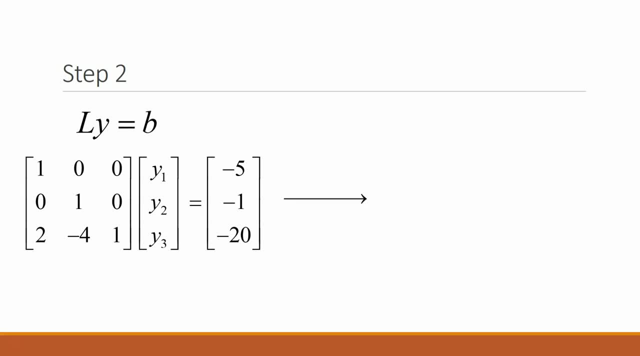 for Y, which can be done by converting the matrices into a linear system. linear system To start solving for y. simplify each of the equations in the linear system. Equation 1 can be simplified into y. sub 1 equals negative 5 and equation 2 can be simplified. 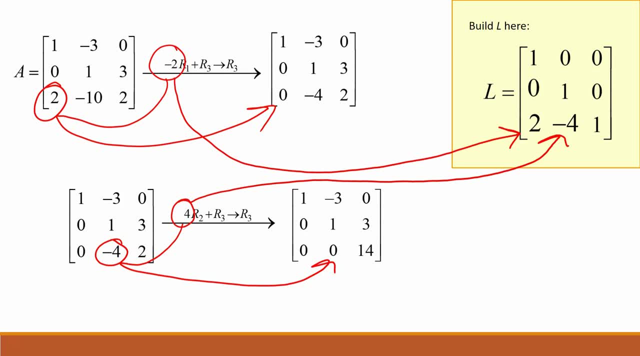 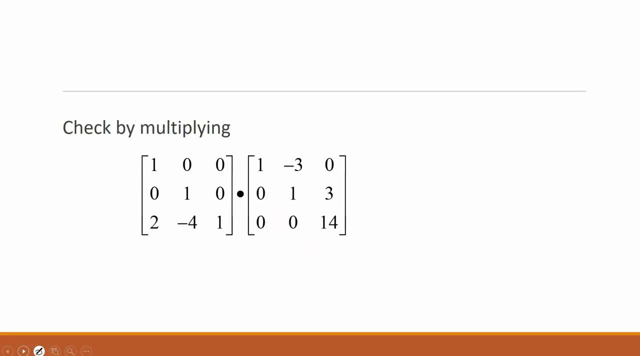 matrix A is now an upper triangular matrix, which we will call U. In order to check and make sure L and U are correct, find the product of the two matrices. This product should be equal to the original matrix A. After a simple matrix multiplication we see the product of L and U is equal to our original matrix A. 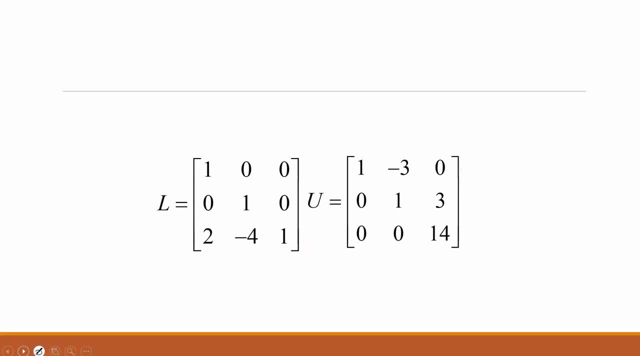 This would be the final answer for the LU factorization of matrix A. LU factorization can be utilized to solve a system of equations. We are given this linear system. If we convert this to a non-augmented matrix, the result is 1. 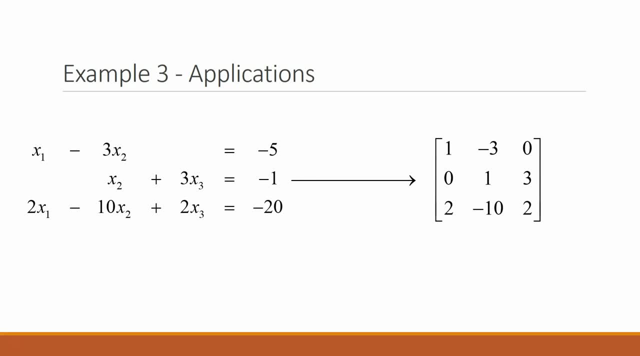 negative 3, 0, 0, 1, 3, 2,. negative: 10, 2.. This matrix should look familiar because it is the same matrix as in example 2.. Step 1. The first step in solving a. 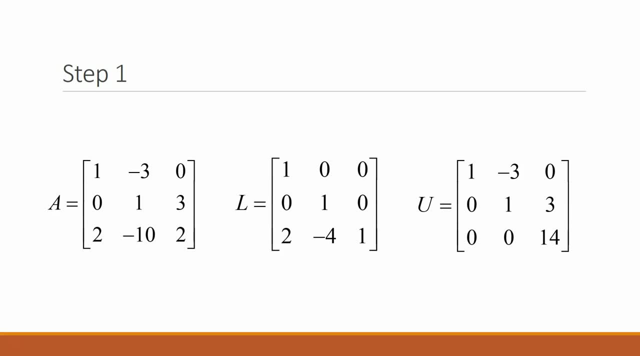 linear system using LU factorization is to compute LU factorization, We factored A in example 2 and these were our L and U matrices which we will use for example 3.. Step 2. Let L times Y equal B and solve for Y. L is our lower triangular matrix. 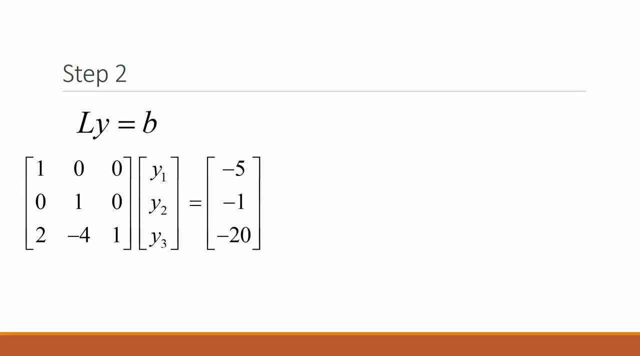 times Y equals B, which are the answers to the linear system. The goal of step 2 is to solve for Y, which can be done by converting the matrices into a linear system. To start solving for Y, simplify each of the equations in the linear system. 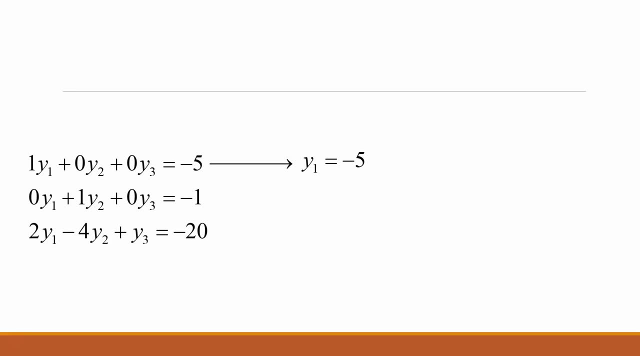 Equation 1 can be simplified into: Y sub 1 equals negative 5 and equation 2 can be simplified into: Y sub 2 equals negative 1.. To simplify equation 3, use back substitution and substitute negative 5 for Y sub 1 and negative 1 for Y sub 2..